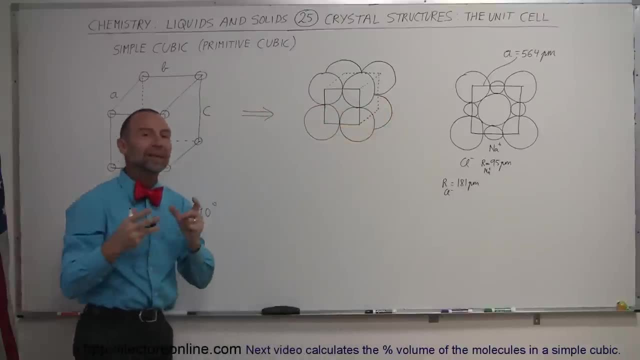 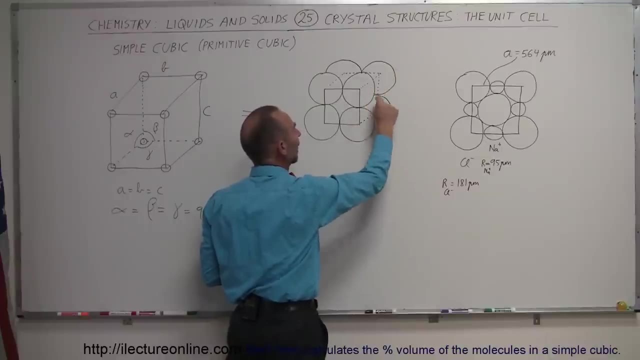 we see that no matter where you put this cube, the content of the cube will be exactly the same. so if we draw another cube right next to it with with four more of these atoms there, you can see that the next cube will look exactly the same as this cube will exactly same as the one to the left, to the 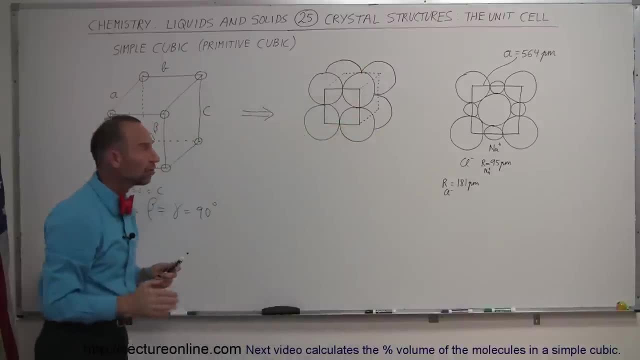 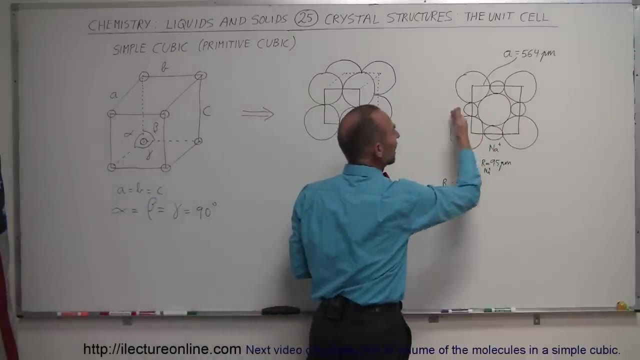 top to the bottom, to the front, to the back and so forth. now, of course, not always are the ions the same shape? most of the time they're not. they're different shape, and so there may be a slight different way in which the atoms are arranged. for example, in sodium chloride, the chlorine atom, the 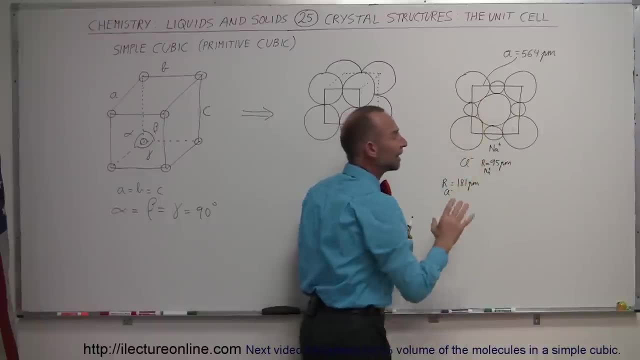 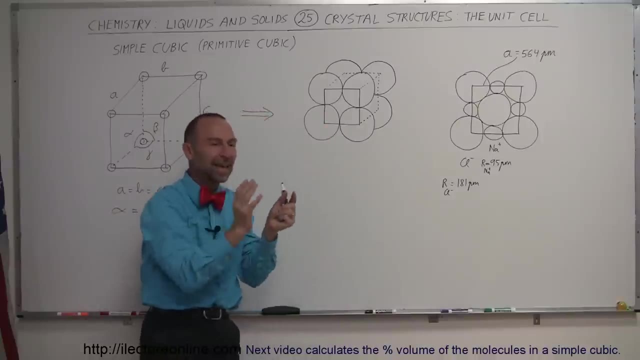 much bigger than the sodium ion, so they tend to pack slightly differently. it's still a cubic shape, but you can see, in order to draw what we would call the unit cell, the cell that represents the same everywhere within the structure has to be drawn a little bit differently. it has to be drawn 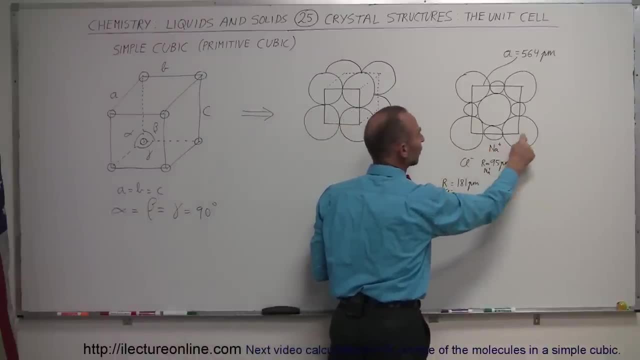 from the center of the large chlorine ion to the center of the large chlorine ion. when you find it again with the sodium ion in between, notice you'll have a big chlorine ion in here, chlorine there, chlorine there. so the unit structure here is a little bit different than it is there, but again. 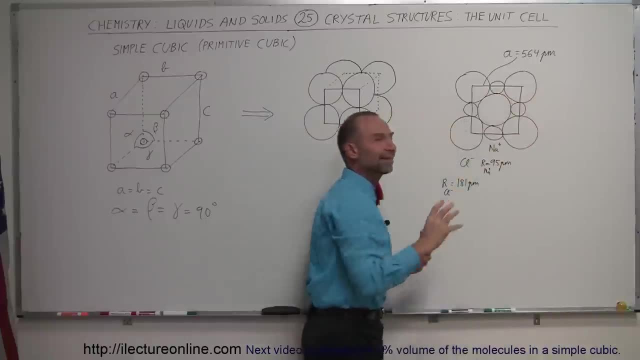 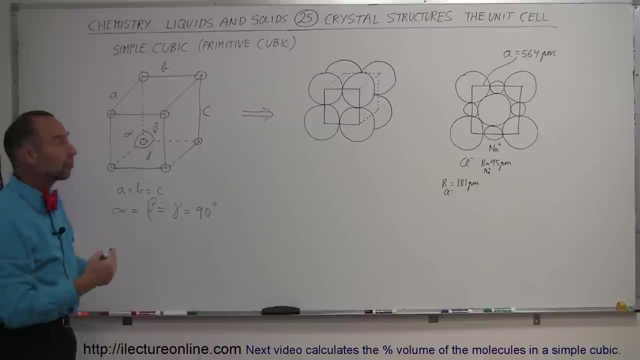 if you take this cube, you place it over here, you'll have the exact same contents of that crystalline structure over there. so that's the concept of the unit cell. so what we're going to do in the next so many videos, we're going to try and figure out what is exactly contained within. 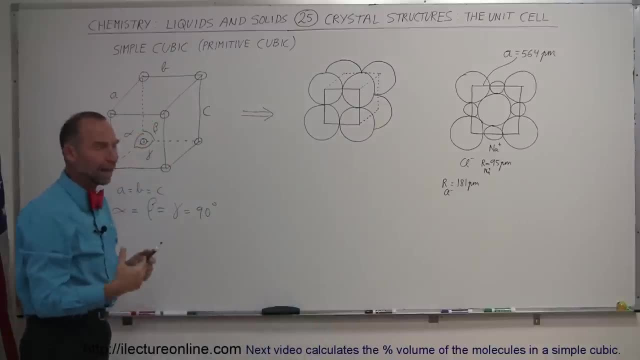 each unit cell, depending upon what the crystalline structure is, what the atoms and ions are involved in the crystalline structure, trying to figure out how much of each atom within the structure is part of the crystalline structure and how much of each atom is part of the crystalline structure. 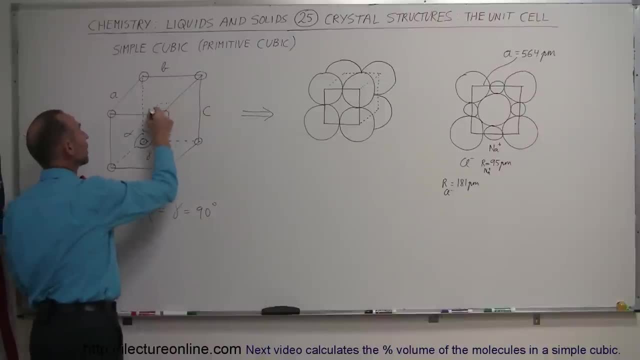 of the unit cell, for example, how much of this particular atom is part of this particular unit cell. and so you may say, well, isn't the whole atom part, or the whole ion part of that cell? no, that's not exactly true, because what we're doing here is putting the corner right at the center of that atom. 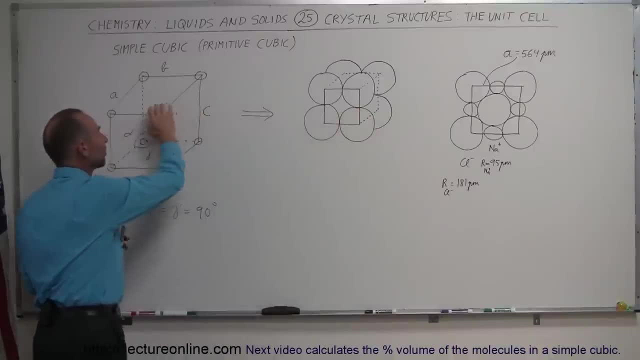 of course, in reality it's more like this rather than this, but sometimes it's easier to see when we draw it out like that. now imagine: there's going to be a cube in the front, there's going to be a cube on top, to the side, and this end at the bottom right here, and it's going to be underneath, to the left, to the. 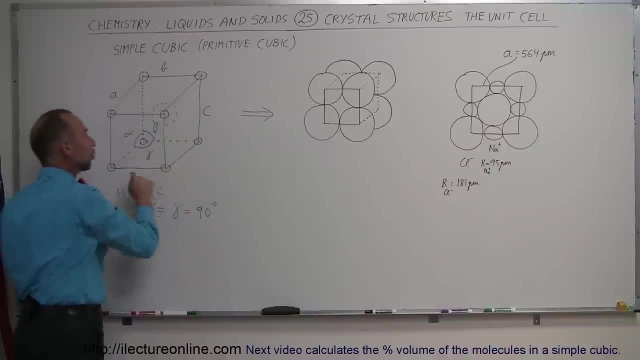 right and so forth, in such a way that each of these atoms of each corner is really shared by eight of these unit cells. only one eight of the atom belongs to this particular unit cell. the other seven eights belong to the other seven unit cells that would be adjacent. 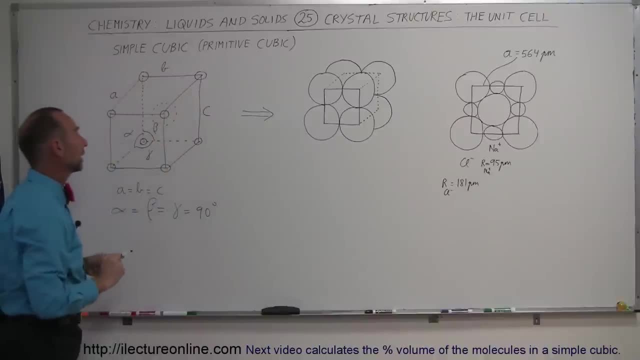 include no encompassing part of this particular atom, like that. so you can imagine: if you draw another one like here, you go straight out. this way you can see that now that this atom is shared between this one, this um, this cell and this cell, if you then draw one in the front this way, in the 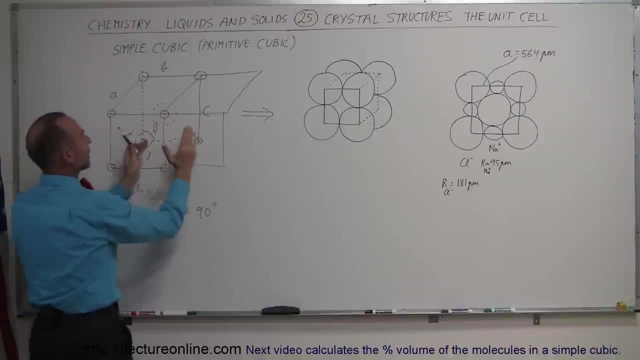 front. that way you can see that this atom is also shared in the unit cell over here and the unit cell over there. so now you have four unit cells here, and so only half the atom belongs to those four unit cells. the other half of the atom would be sticking above those four unit cells. so if you 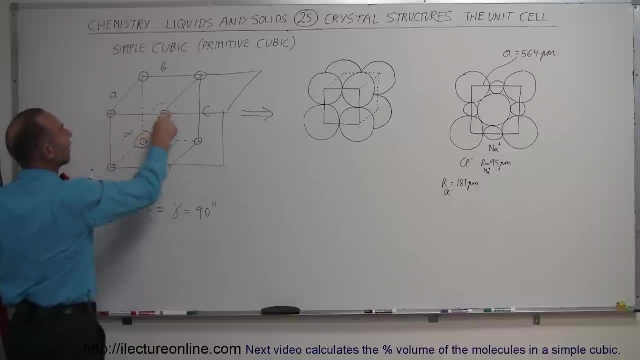 then place on on top of that another four of these unit cells- that's going to be the unit cells- that half of the atom would then be subdivided between those four cells right above it in such a way that one eight of this atom belongs to each of the eight cubes or unit cells encompassing that. 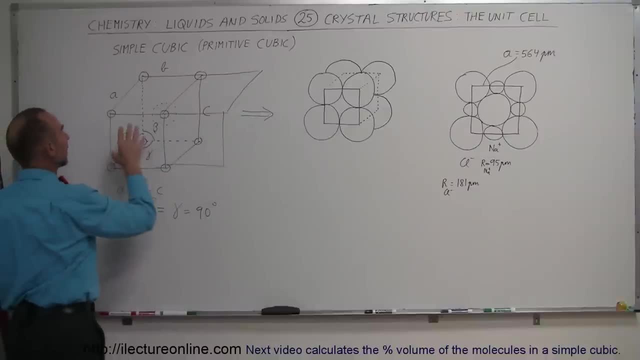 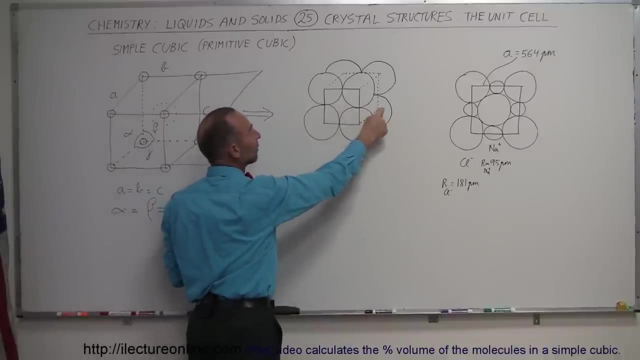 particular region. so how much of the atoms are then inside any one of these unit cells? in the case of an arrangement like this, one eight of this atom would be in the cell, one eight of that one, one eight of this one, one eight of this, one, one eight of that, one, one eight, one eight. and then 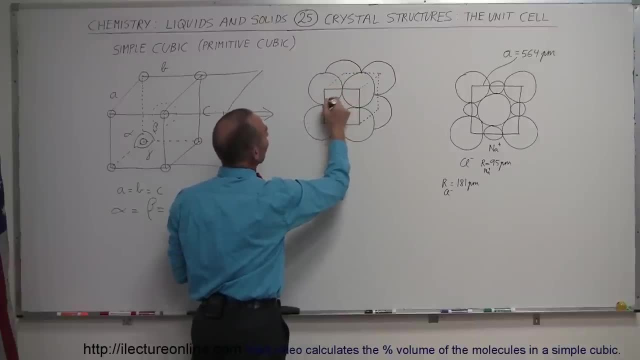 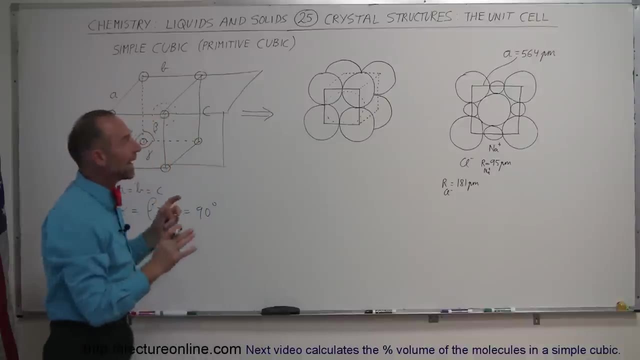 of course there's one in the back here with the other half of the atom would then be subdivided, which i didn't draw. if i were to draw that, it would kind of like sit in the back, like this around the corner in the back of the cube, and so you can see there's a total of eight of those. 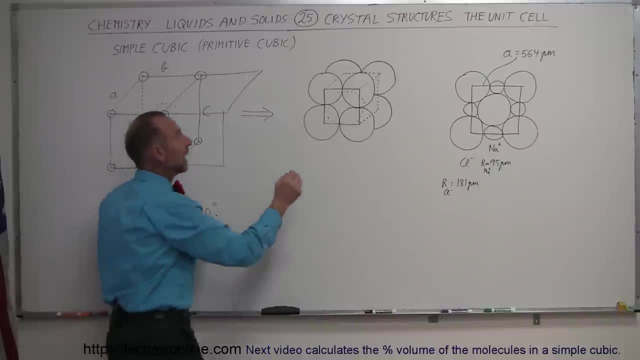 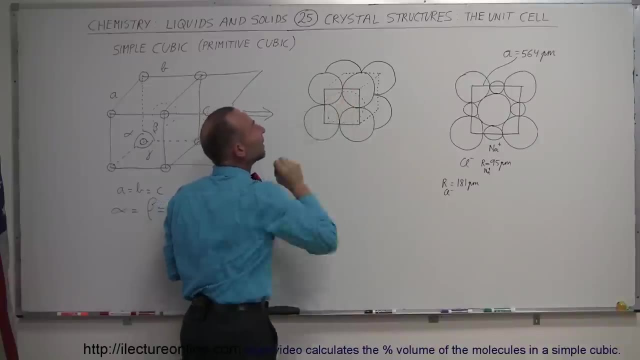 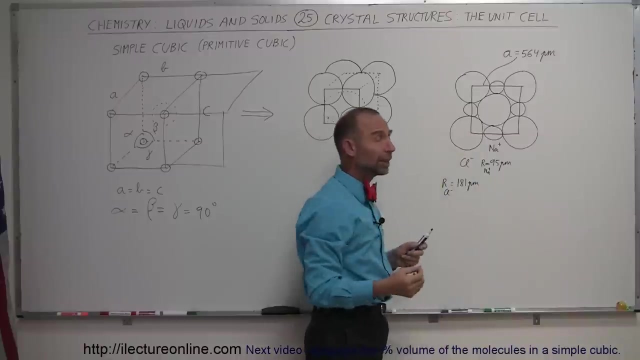 atoms, each of them donating or encompassing one eight of that atom within that unit cell. so this particular arrangement of of atoms or ions would only have one atom within that particular unit cell. as you will see, when we start looking at things such as sodium chloride, which is a little bit more complicated, it's a different way in which you want to count. 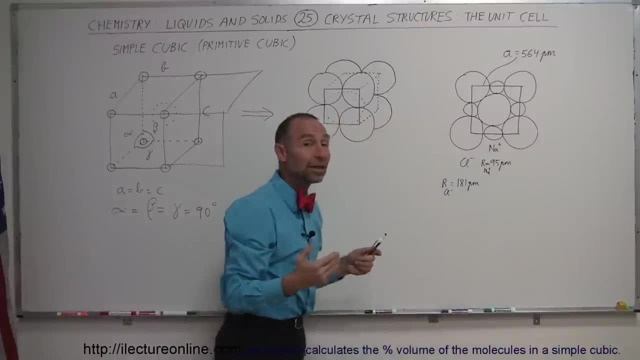 how much of each atom belongs to that unit cell and how you then can find out how many atoms are contained in a unit cell. in a later video, i'll show you how to do that. one thing to keep in mind is that it's important to figure out the size of these unit cells as well. now, for example with 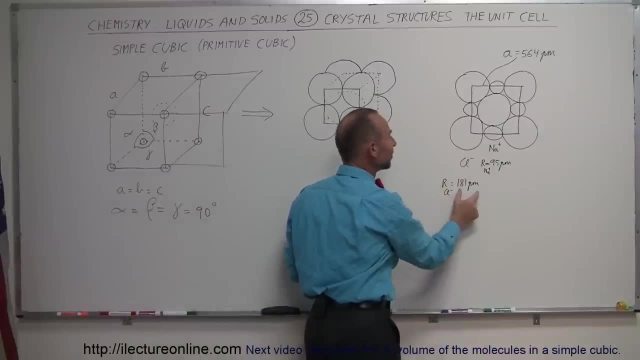 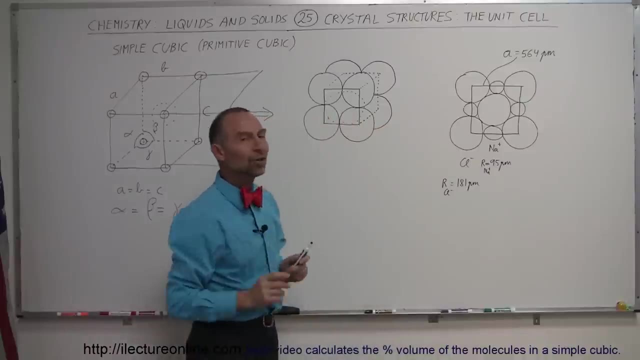 sodium chloride. notice that the the radius of the chlorine ion is about 181 picometers. the radius of the sodium ion is about 95 picometers. so how big is that unit cell? well, through x-ray diffraction techniques we discovered that the x-ray diffraction technique is a little bit bigger than the sodium. 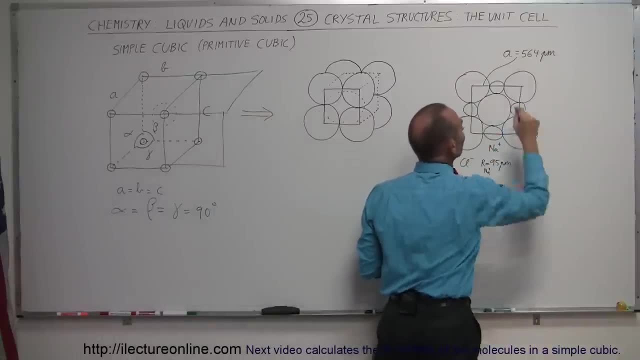 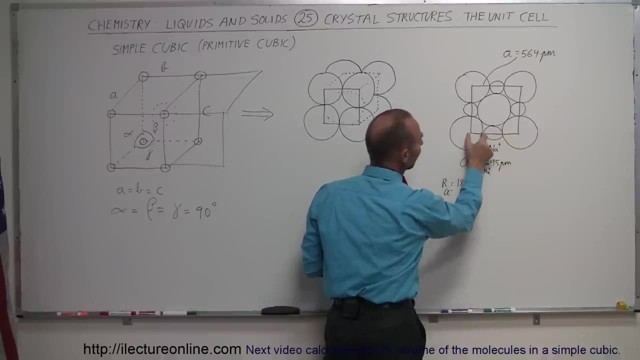 ion. so that means that the unit cell is actually has a side of 564 picometers. now if you imagine for a moment that you would have to take the full diameter of the sodium ion and a half a radius- i'm sorry, half a diameter or a radius of this chlorine ion and a radius of that chlorine and add it all, 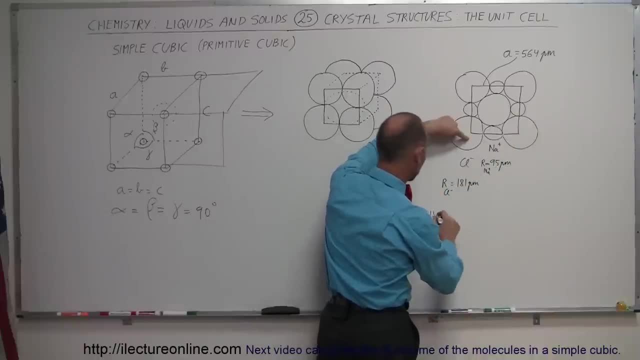 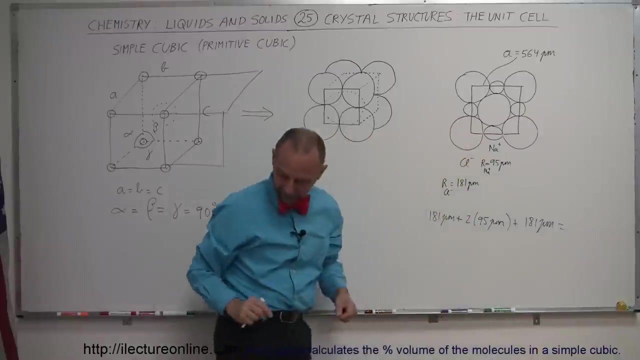 together? what would that add up then up to? so here we have 181 picometers for this, one plus twice 95 plus 2 times 95 picometers, plus then again 181 picometers from that one. and let's see, i have a calculator right here. let's take a quick check here: 181 times. 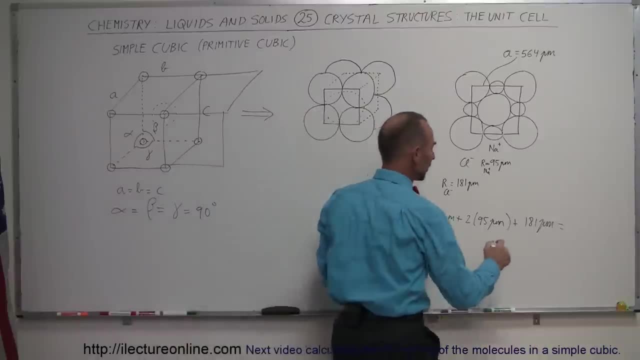 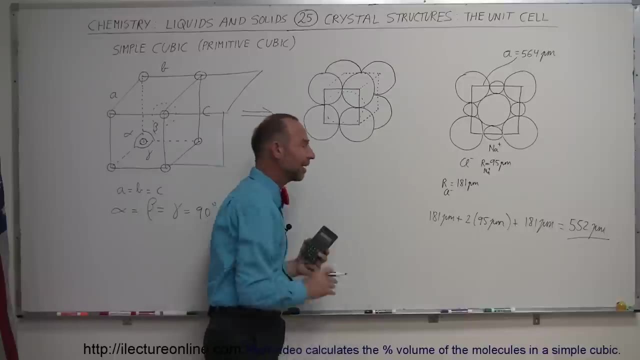 2 plus 95 times 2 equals that would be total of 552 picometers. so from simple calculation and knowing the average size of these ions, you would expect the unit cell in this case to be 552 picometers on each side. in actuality it's a little bit more, it's 564. 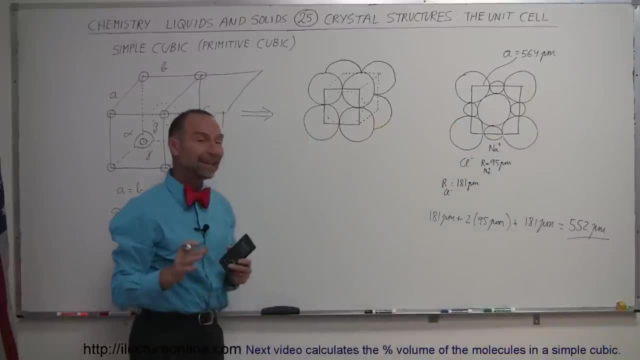 picometers. so why the difference? well, it turns out that these are average values for the radii of these particular ions. depending upon what they're mixed with, that radii can change. that, of course, it involves electrical electrical forces, and so sometimes they're squeezed a little bit closer. 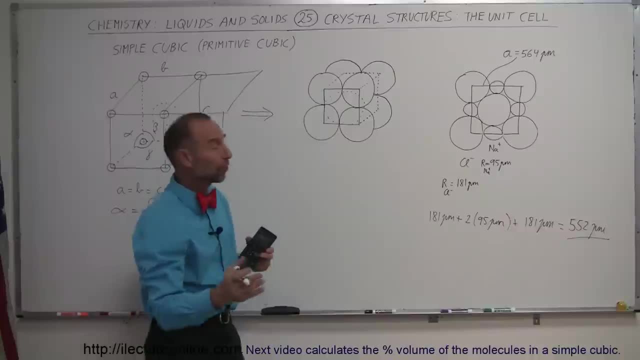 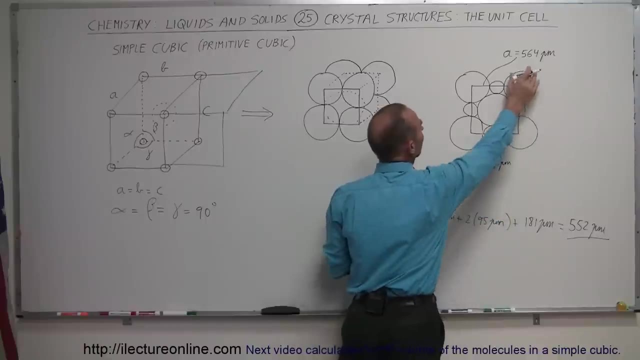 together. sometimes they're repelled out a little bit further out and in the case of the sodium chloride, notice that the close proximity of the chlorine ions probably pushing designs a little bit further apart so that the unit cell has a sideắnon of鬼. 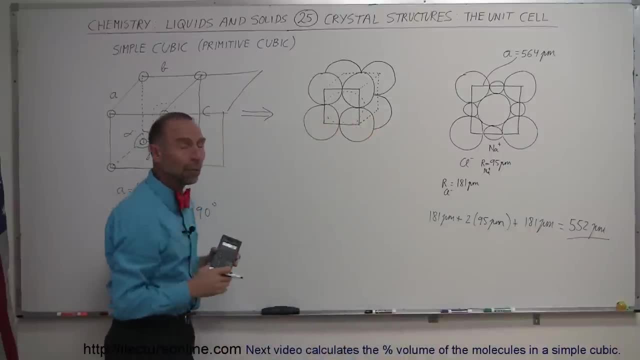 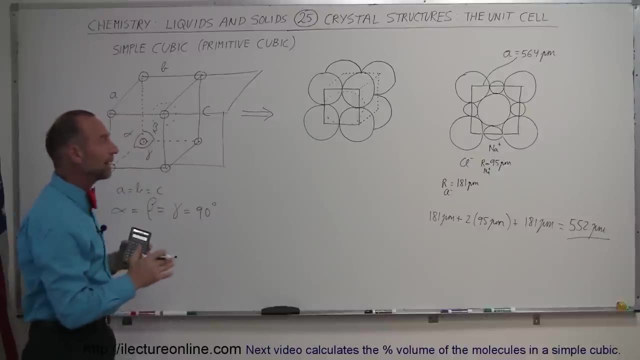 distance or length of 564 picometers, rather than what we would expect to be 552,, but it's in pretty close agreement. So that's the basics of the unit cell in the crystal structure of atoms in the solid state, and now we're going to systematically look at the various types of crystal structures. 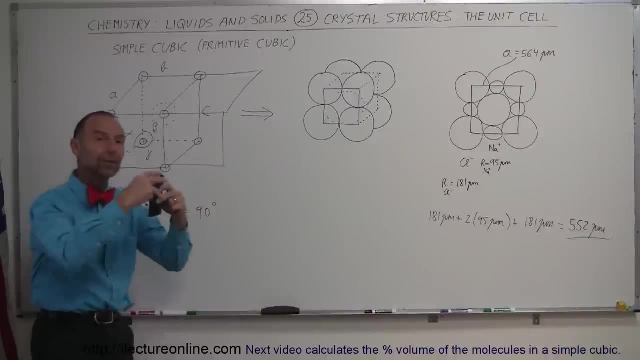 that can exist and the various ways in which atoms are packed with those crystal structures, and from that we can calculate densities and so forth, and that's a pretty neat thing. So stay tuned. take a look at the other videos if you're interested in this kind of stuff.